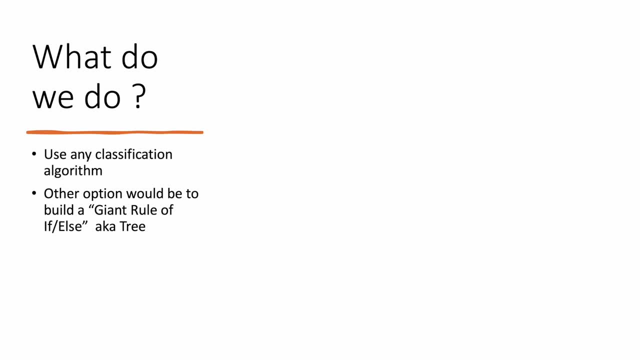 a statement. Why do I mention, if else, a statement? We'll try to see that in a moment. This is how a decision tree works. If you are coming from a non-computer science background, this would look little weird to you. This is actually an inverted tree. if you see, The top most is is the root and 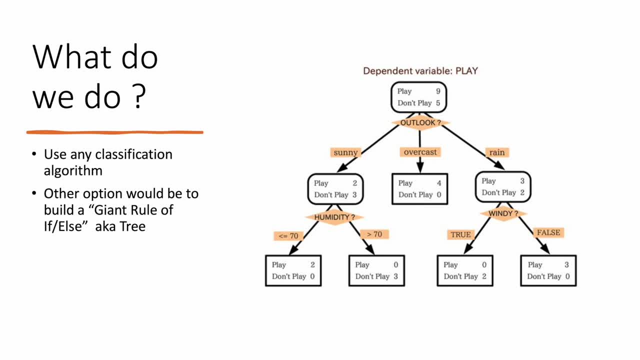 the bottoms are the leaves. In a natural biological tree, it's the other way around: Root is at the bottom, The leaves are at the top, but over here in computer science, it's the other way around. right, This is a tree, This is a decision tree. Now, if you notice this decision tree, My first decision, I'm 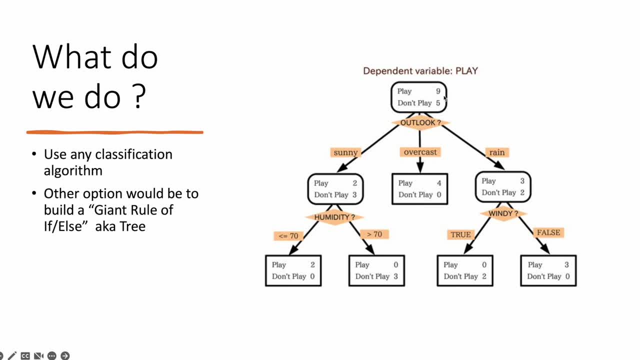 making is that, whether the outlook, if you see the play nine and don't play, these are the observations. So I have nine observations where I'm playing and five observations where I'm don't playing. Now, based on outlook, whether outlook is sunny, overcast or rain, I'm further splitting it. 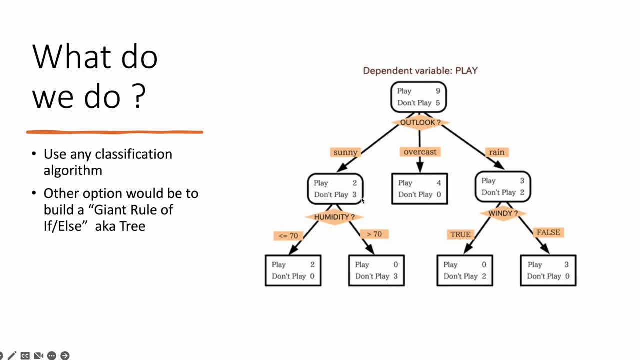 This is nothing. but if sunny, play two, don't play three observations. If overcast, play four, don't play zero. If rainy, play is three observation and don't play are two observations. So this is a two observations. over there, If you read this, let's say on the right side of the tree it reads: 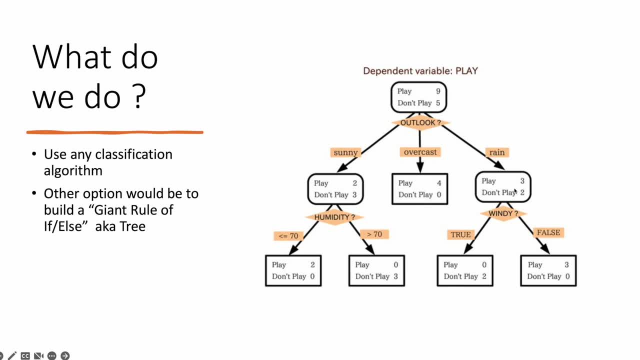 like if outlook is rainy and windy is false play, because the don't play observation becomes zero, So this becomes a leaf node. over here, The majority class is for playing, not don't play, So my vote will go, or my prediction will go, to play. That's the reason why I'm saying, friends, that this is. 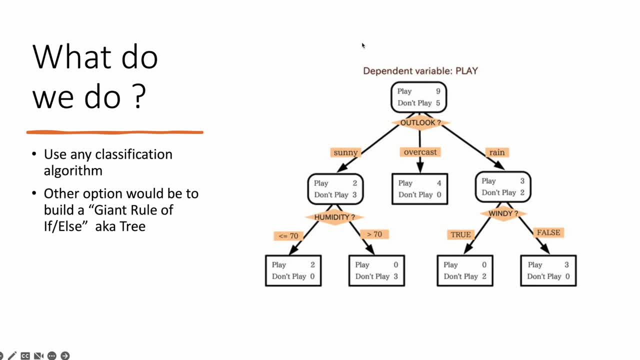 giant rule of, if else a statement, Again repeating: if outlook is rainy, if windy is true, don't play right. don't play will come to two right. So this is in nutshell what decision tree is. Now we'll try to understand how to build that. It looks very easy, nice and clean, but how to build that There? 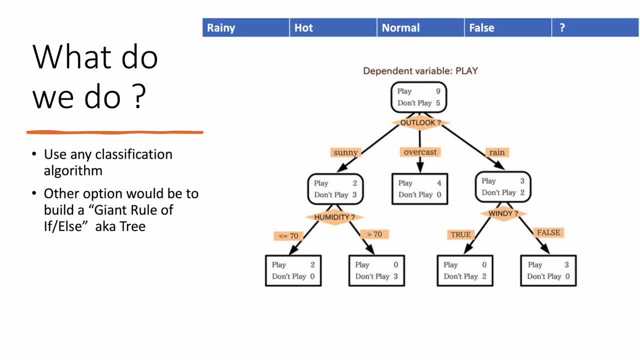 is a science behind that. We'll try to learn that, okay, Now to give you the example, the or. what we did was: if it's rainy, hot, normal and false. if it's rainy, the red arrow. if it's false, okay, windy is false. we are not using the use of the middle two features. then I should go and play my prediction. 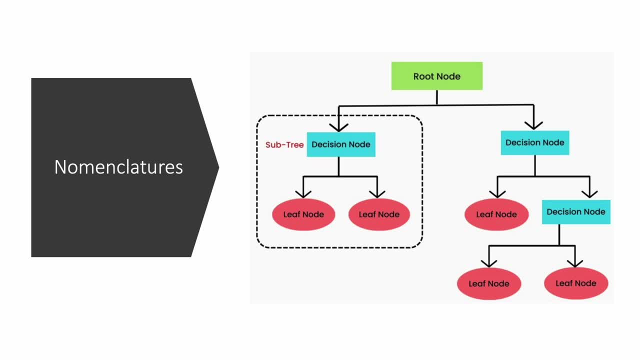 will be play right. Let's try to understand few of the nomenclatures because before we dig deeper into decision tree, As I was saying, the root is at the top, so it is called root node. The other is the. it is windy, true or false, outlook is sunny, cloudy, that is called decision. So after root node, 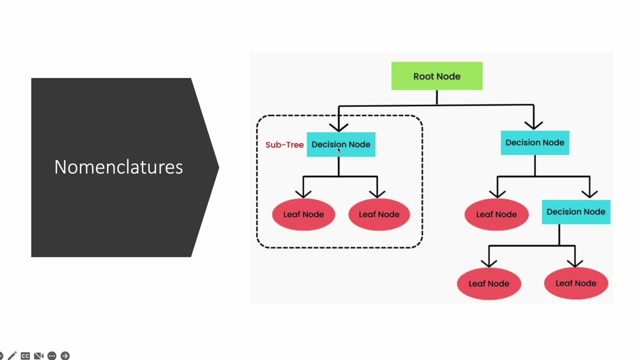 there will always be a decision node. Decision node is nothing, but where we are branching out whether we are making a call, whether it's true or false, less or more, greater than or smaller than right. We are taking an, if else a statement over there. that is the decision node. Similarly, this: 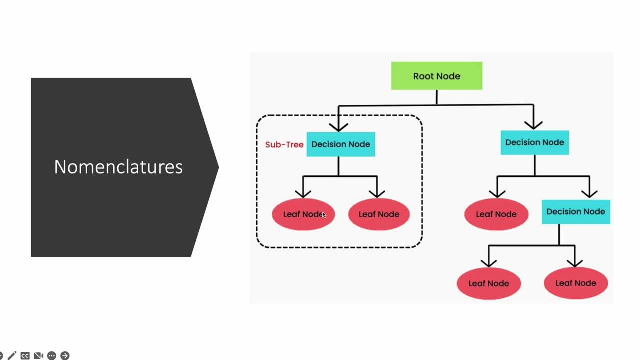 will keep branching out. okay, The portion where the it stops branching out is the leaf node Is the end, and of the tree is the leaf node. Now, there can be multiple leaf node, but there will be always be one root node, right? this whole thing is called a tree and a similar structure is called 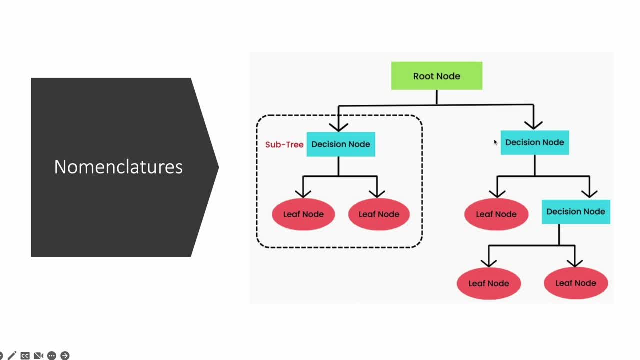 a subdree. So if you see in the dotted this is a subdree on the right side Also, this whole thing is a subdree. this particular thing, anything which is decision node and in everything beyond beneath that Can be termed as a subdree. So 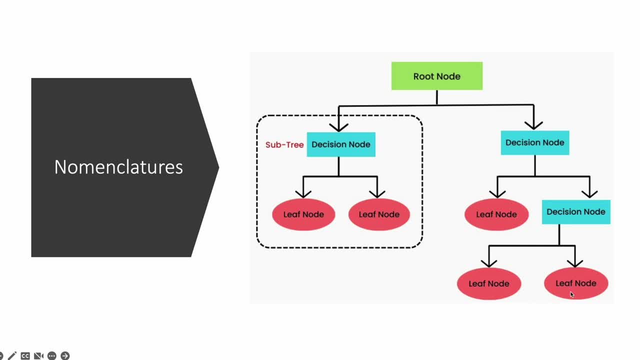 This can also be termed as a subtree. This particular whole thing can be termed as a subtree. So this is a right subtree for this root node. This is a left subtree for the root node. Now we understand what is root node, what is decision node, what is leaf node? 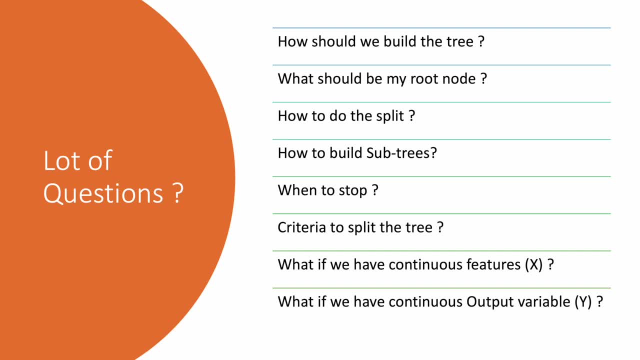 Let's move on. But there are a lot of questions. We understood that. okay, how intuitively decision tree works. It's a if-else statement and all those things. But how should we build the tree? What should be my root node? 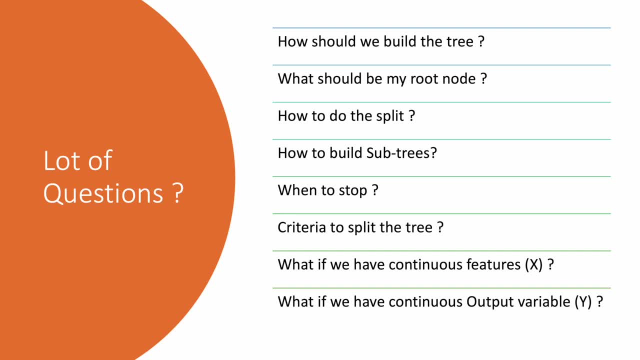 As I was seeing, there were four features. Which feature I should pick for my first decision? node, right at the root, at the very root, How we should do the split right. If there is, let's say, outlook is sunny, windy, sunny, cloudy and rainy, how should we do the split? 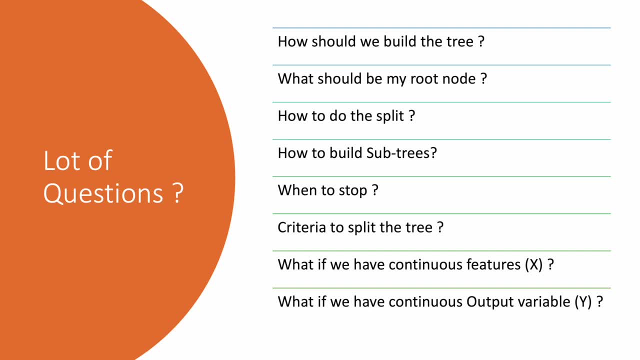 Again, if we make the root node, how should we make the subtrees? What is the logic for making the subtree? What is the logic for making the subtree? When to stop, Do we always need to go to the leaf node? How will we know that we have reached the leaf node? 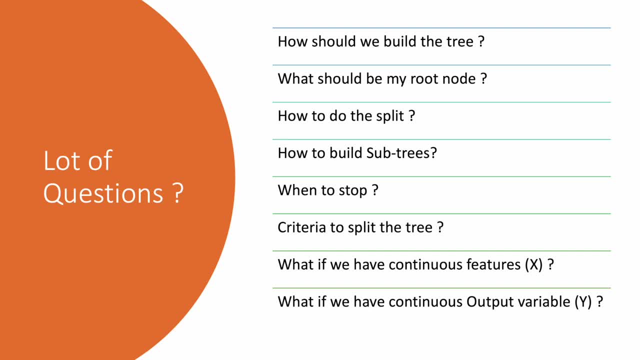 What is the criteria to split? What if we have a continuous feature x? So one of the feature, or many of the features are continuous variables. right, Instead of categorical. which is sunny, cloudy, rainy, if suppose it's a number like temperature. 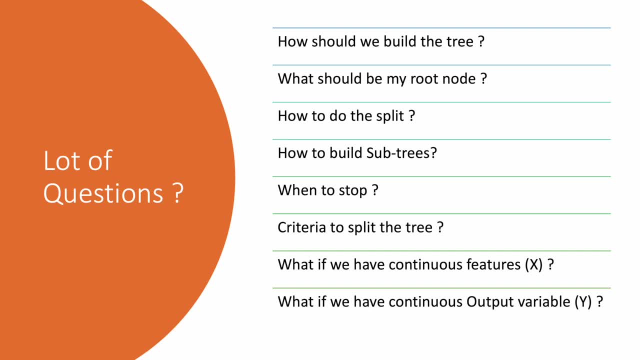 Temperature is not given between high, medium and low. It is given like 17 degrees centigrade, 24 degrees centigrade, 13 degrees centigrade. That's a continuous variable. So if my feature is continuous, how should we deal with that? 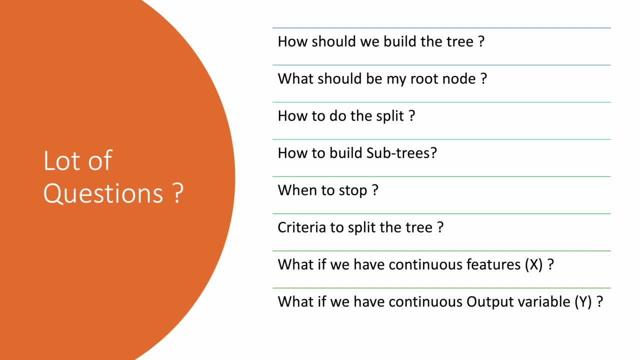 What if my output variable y itself is continuous? What will happen then? If my output level is continuous, that means it becomes a regression problem. So rest, all the things are related to classification, which applies as well to the regression setting. But the last question is specifically if you are asking that: hey, what if my feature is continuous? 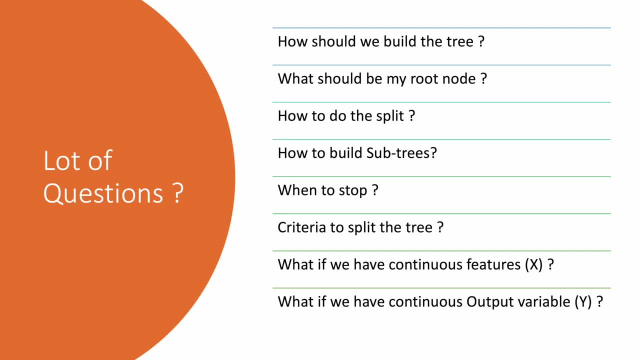 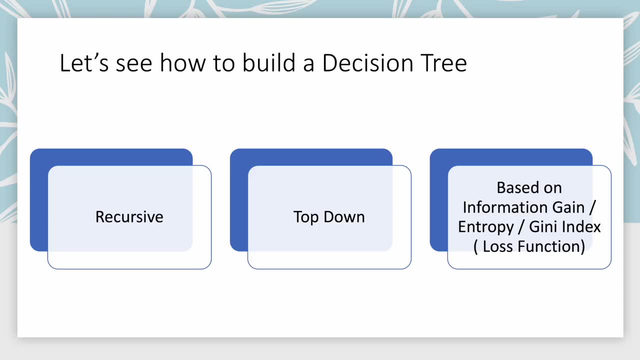 What if my output variable y is continuous? It becomes a regression problem. Let's try to answer each of these questions and understand decision tree in greater detail. Let's see the first question. Let's see how to build a tree. So we have three principles to build a tree. 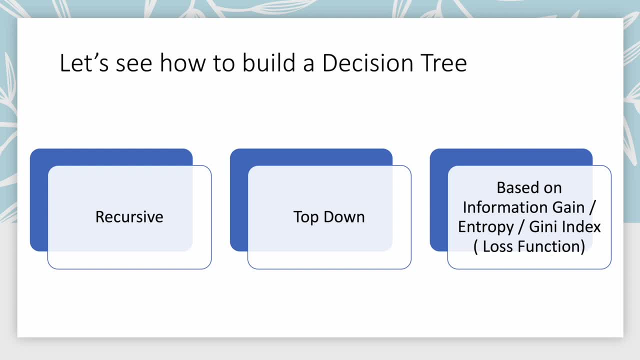 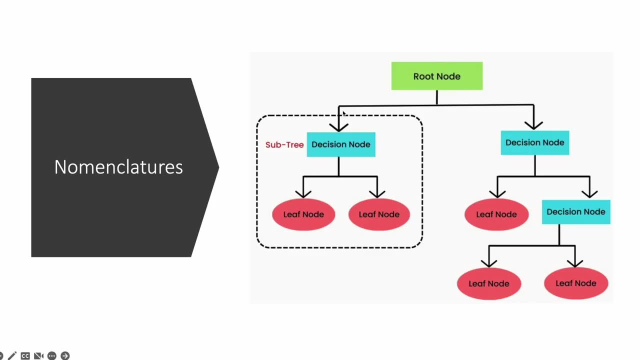 One is recursion. We recursively build a tree. By that what I mean is: let me show you: So we build the root node, We do a split over here To build this particular tree. I will use a recursive logic, what I have done for splitting the root node also. 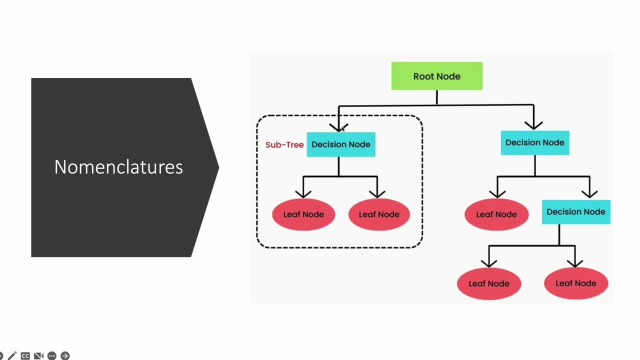 So I will write my logic one time and the same logic I am going to apply To build this subtree for this subtree. it will look as if this whole subtree is a complete tree in itself. That's the way we will do And that's the meaning of recursion. 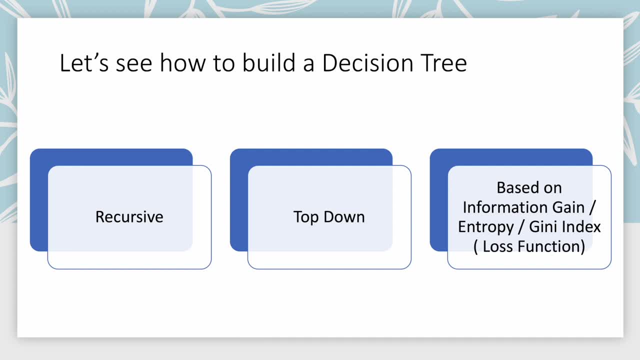 Recursively. What is the meaning of top-down? Now you are saying that this is an inverted tree. right, In computer science we will always look at inverted tree. So we will start from the root. top-down, That means start from the root and then branch out to subtrees, further subtrees, further subtrees, till we hit a root node, a leaf node. 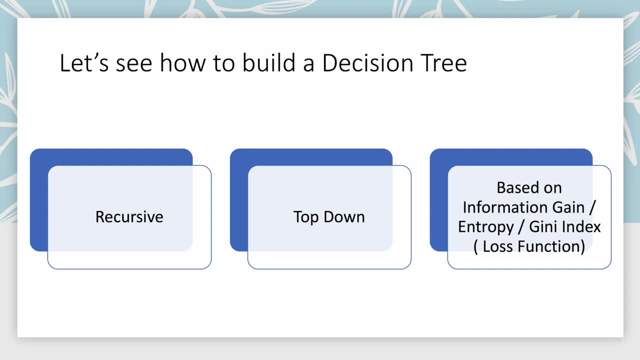 The third thing is: how do we do the splitting? We do the splitting based on the principle of information: gain, entropy, Gini index. These are big terms. We will just explain that in a minute, But try to understand at a fundamental level. 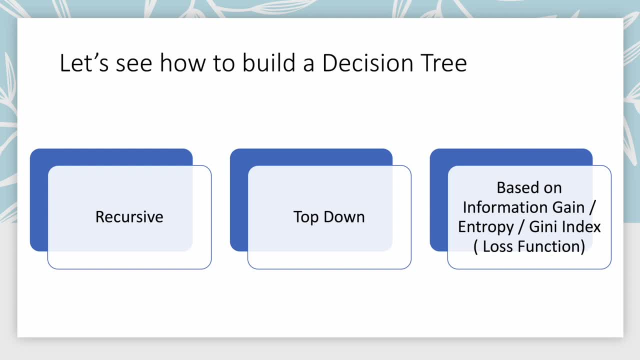 Decision tree is also a machine learning algorithm And, like any other algorithm, it has to have a loss function which we have to minimize, which we have to optimize. In case of logistic or linear regression or SVM or any other naive base, there was a loss function which we are trying to minimize. 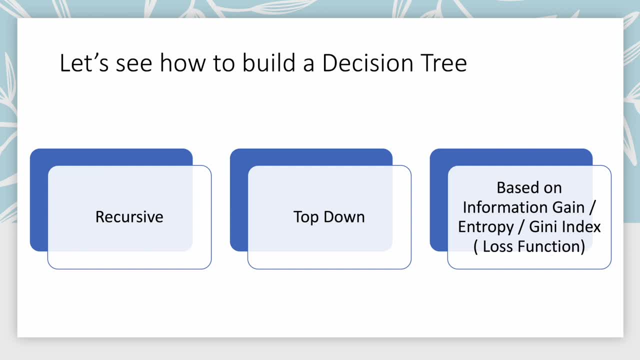 Right. So what is the loss function in this particular case? What is the thing which we are trying to minimize? to build the tree recursively? Okay, That particular thing is entropy, Entropy. we are trying to minimize the entropy. We will just see that. what is the definition of entropy? how we measure entropy. 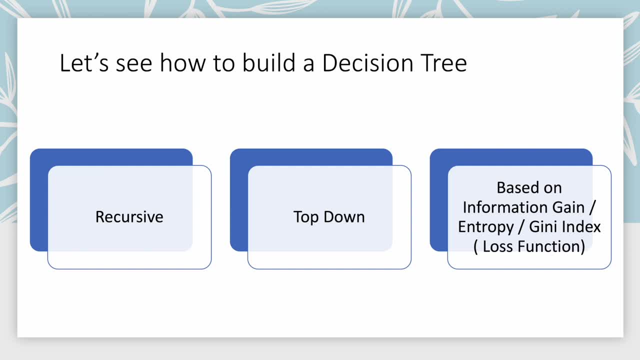 But try to understand that this is something. this is like my objective function, which we are trying to minimize, Or my loss function, or my cost function, which we are trying to minimize to build the tree recursively. Okay, Let's move on. 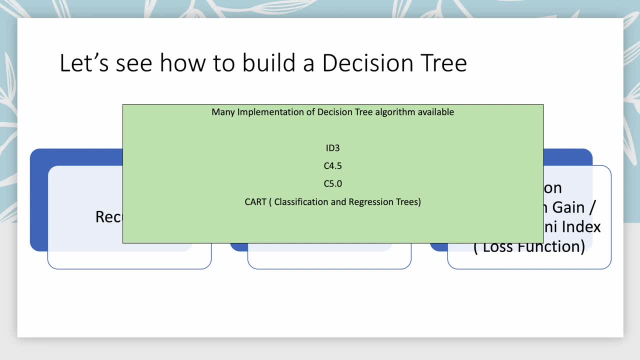 Now, one thing I would like to mention before moving forward is that there are many decision tree algorithms which are available. Right, So you will hear names like ID3, C4.5, C5.0 or CART. CART is the classification and regression tree algorithm. 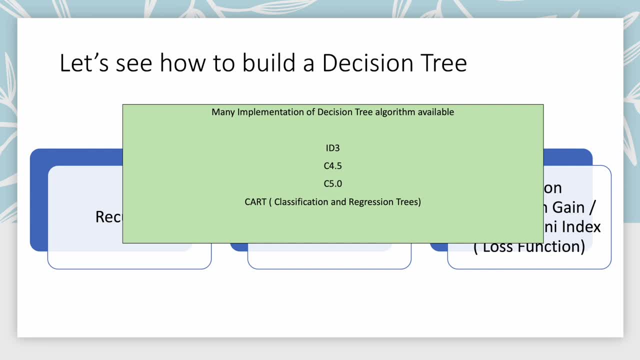 This is one of the implementation of decision tree. Okay, CART is the algorithm which scikit-learn package also uses. Okay, So we will devote our tutorial to specifically talk about this CART implementation of decision tree algorithm. Now, one of the key differences over here is that CART implements binary tree. 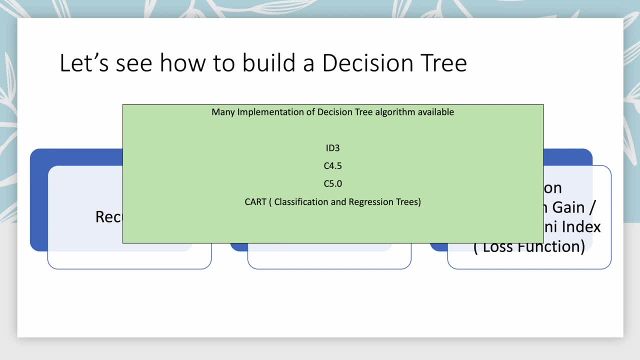 Binary tree means friends. if you recall, the outlook was sunny, cloudy and rainy. Right, There were three classes. But in case of CART algorithm, which scikit-learn package, Which scikit-learn implements also, Every node will branch out into two. 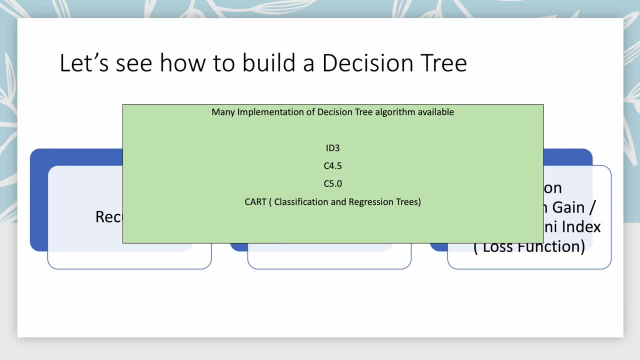 So there has to be a yes- no answer Right. It cannot be yes, no and maybe Or multi-class or multi-label problem. It cannot be like that. It has to be a yes no. Greater than seven, less than seven. 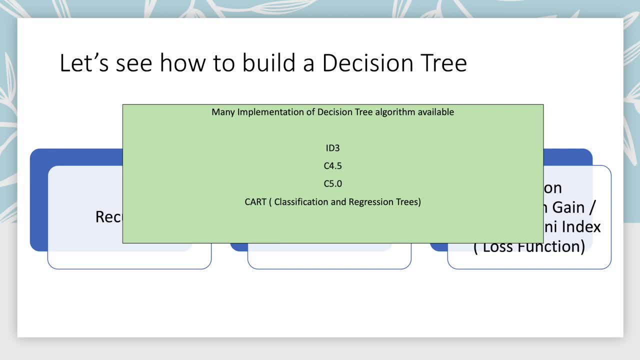 Is present, not present Right. Those kind of situation has to be there And we will see that If one of my feature is suppose multi-category, Right, So there are three categories over there. How can we convert that problem into a two category problem? 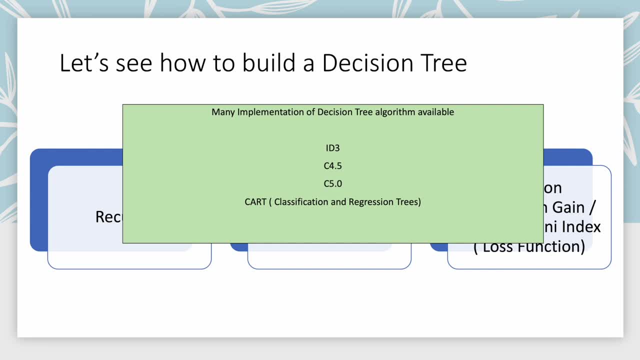 We will just see that Right, But from the time being, let's understand that we are going to learn about CART, And CART is the thing which is being implemented by Python scikit-learn package- Okay, Which is tremendously used, But there are other implementations also present in the market. 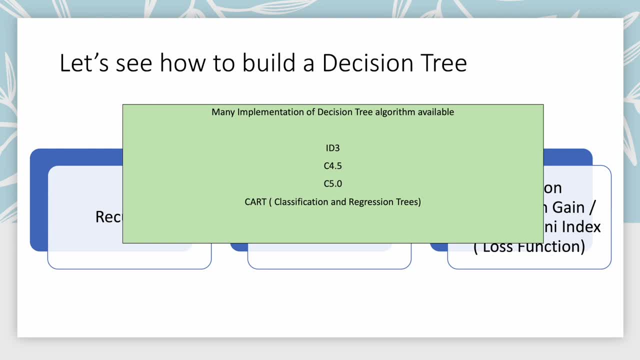 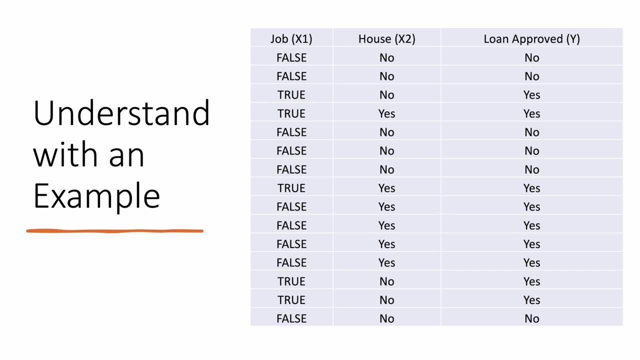 Like ID3, C4.0.. ID3, C4.5 and C5.0.. Okay, Let's move on. Let's understand this with another example in a further, greater detail. Right, Okay, This is my data set. 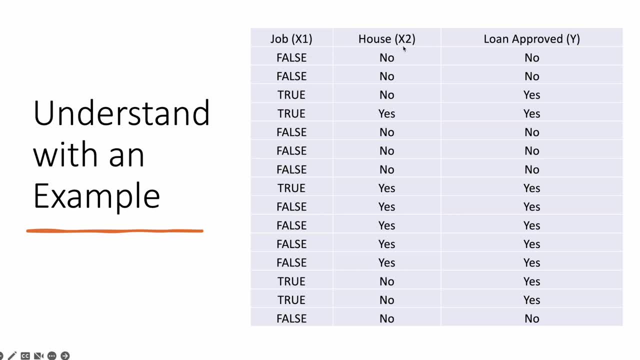 The data set is very simple. It has two features, X1 and X2 over here, And one Y variable which is loan approved. So this data set is that, whether the loan should be approved or not, I am building an application which will predict the loan should be approved or not. 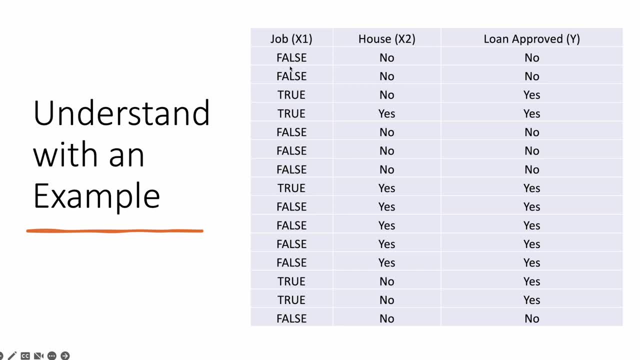 And this is the feature of the person who is applying the loan. So the job: whether the person has a job or not And whether the person has a house or not. Based on these two simple criteria, categorical criteria or features, I am going to predict whether the loan should be approved or not. 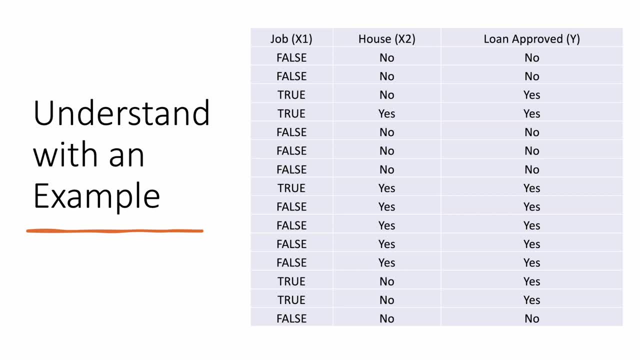 Very straightforward data set And we will try to implement decision tree based on that. Now we can always convert this into 0 and 1.. Since this is a binary, my binary classification, my Y, is also yes and no. There is no, maybe over here. 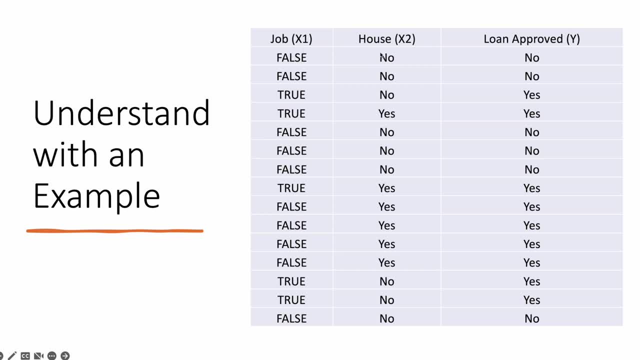 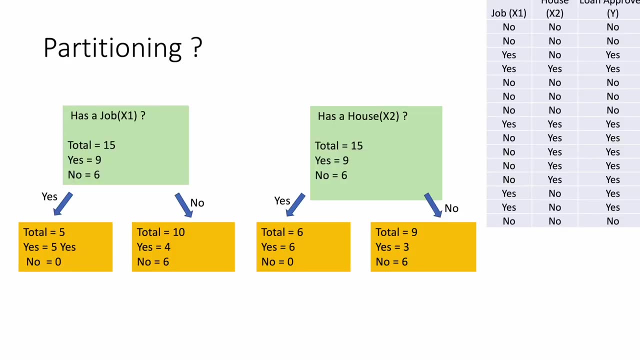 And if you notice my job and house, both are binary categories, Right? So either true and false, yes and no, We can easily convert that into numerical 0 and 1.. Right, Okay, Now let's see. If you recall, our first challenge was: hey, how do I select a root node? 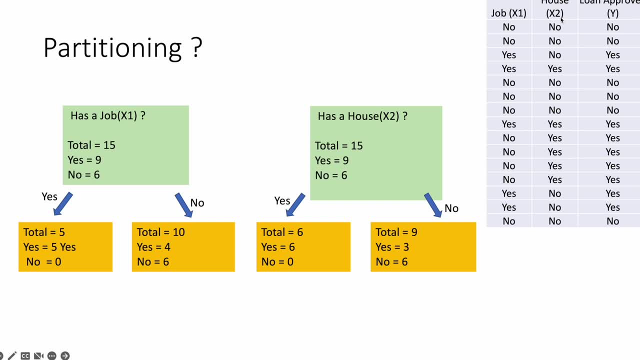 Now, if you notice, here is X1 and here is X2.. Right, So we have two features over here, Right, Job and house. Which feature or which decision should be my root decision? Right, That is the question. And now, once we understand that, then recursively we can build the rest of the tree also. 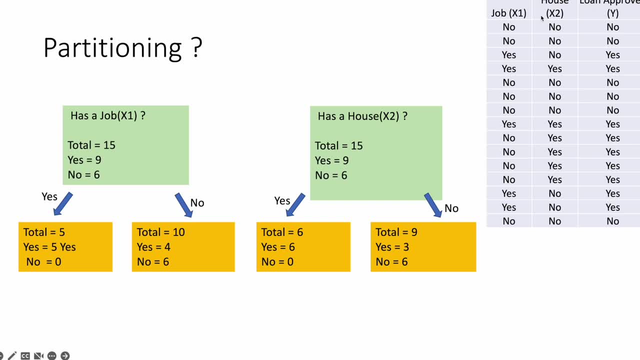 Now let's try to understand how the first split happens, The root split, how that partitioning happens. Let's say what decision tree says: is that you try to do the split on both of them Right? Both of them are a candidate, the job and the house. 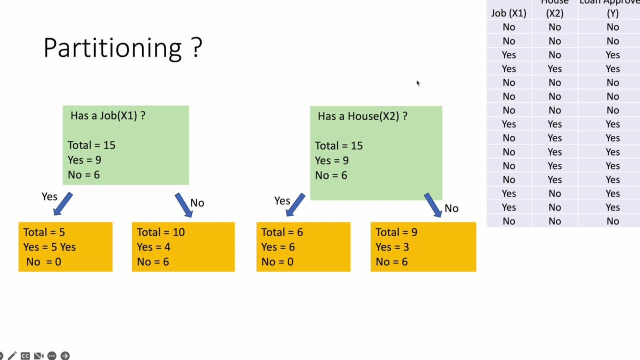 We'll try to split on both, on job and house, And we'll try to see that what's happening. Okay, Now, the first decision was, or the first point of the split was: has a job X1.. So total how many features we have. 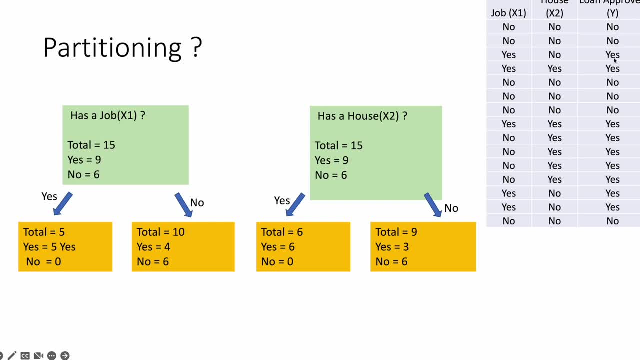 15 features. How many? yes, we have 9.. How many no? we have 6.. In case of house also, it will be the same thing, because we are at the root node Right Now. let's see, Okay. 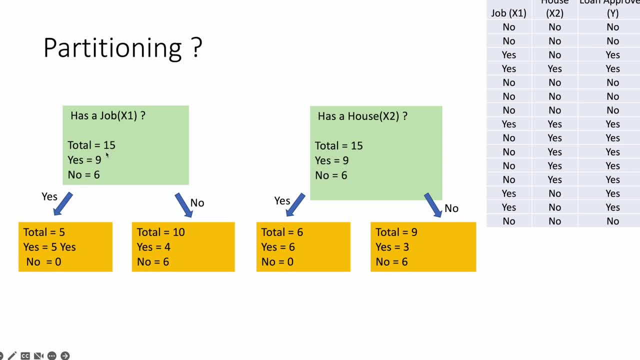 If I'm splitting on the base of job X1. Right: Job is there or not. Job is yes. That means this feature, this feature, this feature and this feature Right. These observations- sorry If I have these observations. 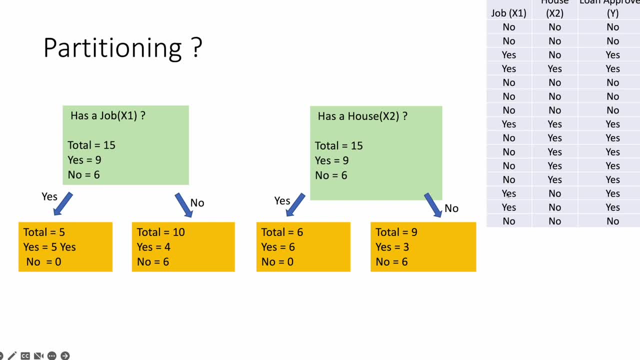 Now, if there are the observations, how many observations are there? 1,, 2,, 3,, 4,, 5.. 5 yeses: How many total Total? Now, if I do yes on my left side, on the yes side, how many observations fall? 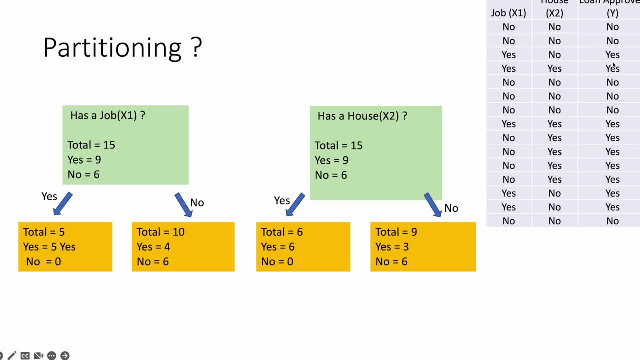 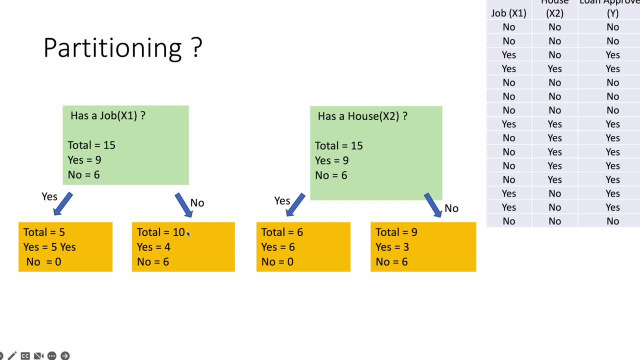 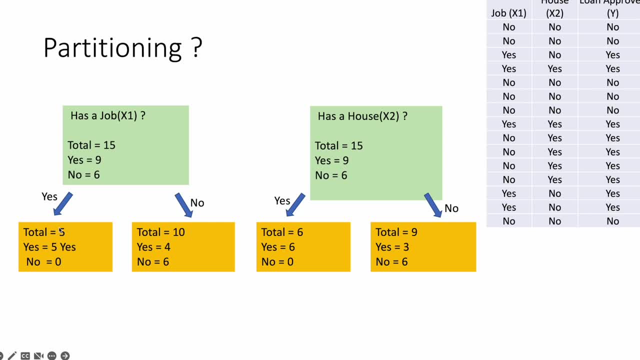 Right. So overall we have 5 observations went on the left side. 10 observations come on the right side with no Right Out of those, how many yeses are there on the Y side: 4.. How many noes are there on the 6?? 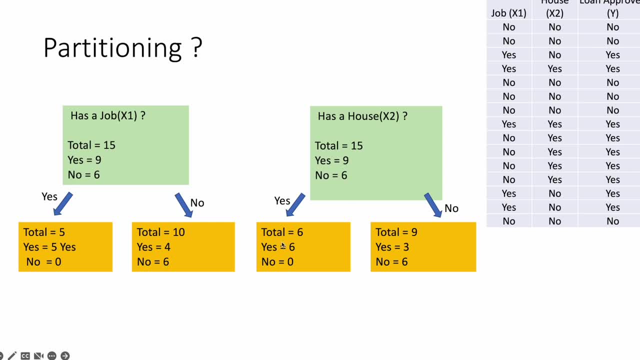 Right. Similarly, we will split this also Now. you will ask that why we are doing this split. Now just wait for a minute, and before let me explain this. So let's try to see again. I am repeating how the split is happening. 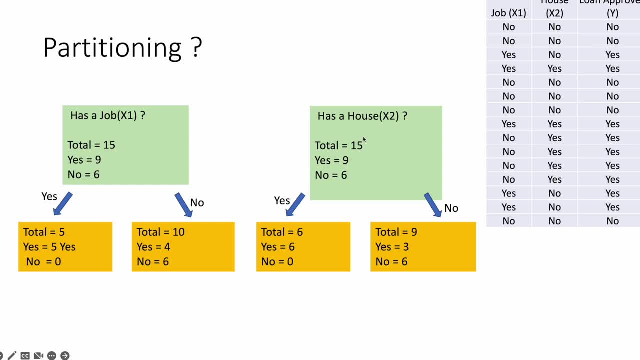 Split is happening. Both are candidates. We are trying to split on both of them And out of these two we will select one. split Right- Either job or house, because we have two features. If we have M number of features, there will be M number of candidates. 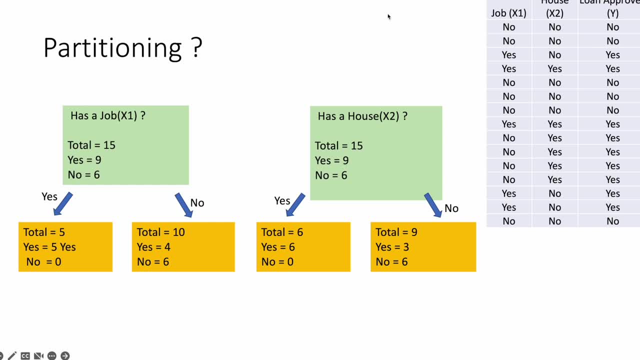 And we will try to do this exercise for all of these features. Right, And how we are doing this exercise. We are trying to split this into yes or no, Or it could be like low or high. whatever be the category, We are trying to do the split. 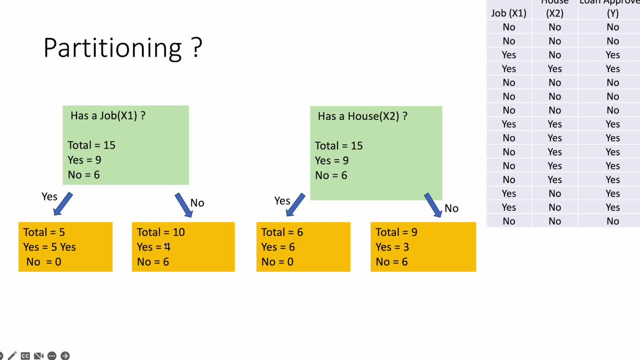 And then we are counting the number of in each of these buckets after the split. we are counting the number of how many total observations were there, how many of those were yes, how many of those were no Right. This is based on the Y- predicted Y variable. 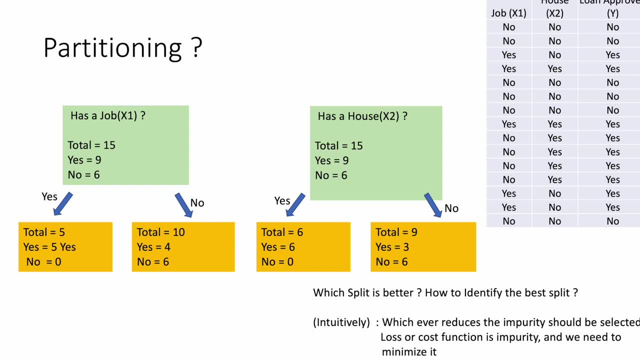 Right, This is what we have counted till now. Now, if I ask you that, hey, should I do the split on X1 or X2?? Which one is better? There is no way of clear knowing that. Right, We have to quantify this information, that which one is better? 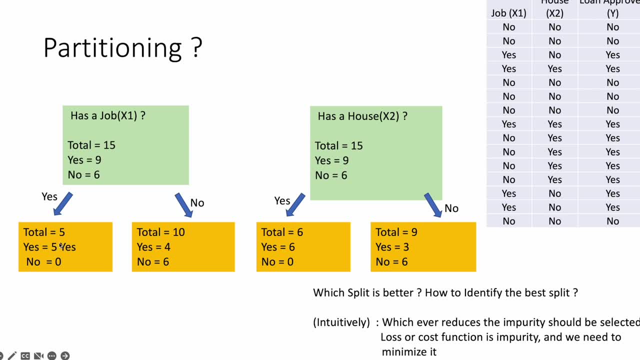 Intuitively, it makes sense that hey, looks like this: 5, 0.. Okay, This is a cleaner split, Right, Cleaner split. What do you mean by cleaner split? That means over here. here comes the concept of entropy. 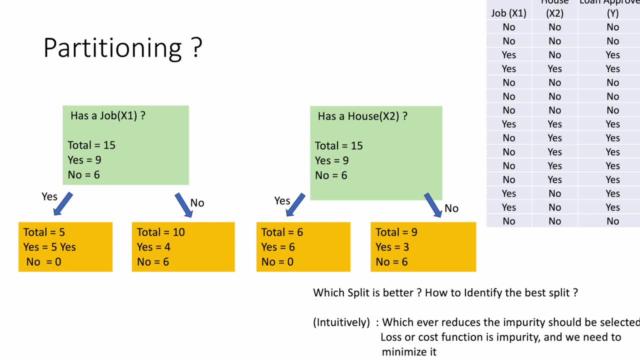 Entropy is a concept which came from physics But in machine learning and computer science it is used in information science as well, And it says that the amount of impurity present in a particular data set Right. What do you mean by impurity? 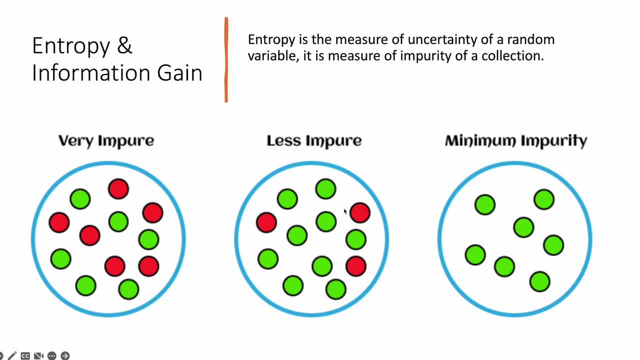 Let's try to understand that. Let's try to see this particular picture. So there are green circles and red circles. The first picture is saying: very impure Entropy is very high in the first picture Why? Because it's like half half. half is the red, half is the green balls over here. 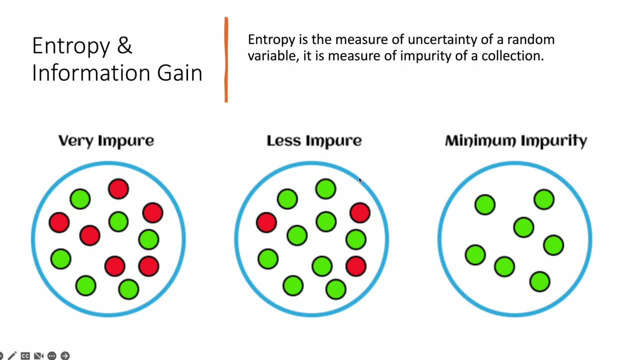 This is less impure. Why this is less impure? Because, if you see, the red balls are very less compared to green balls. Okay, This is almost pure, or actually pure. This carries the minimum impurity. Why? Because there is only one class which is present. 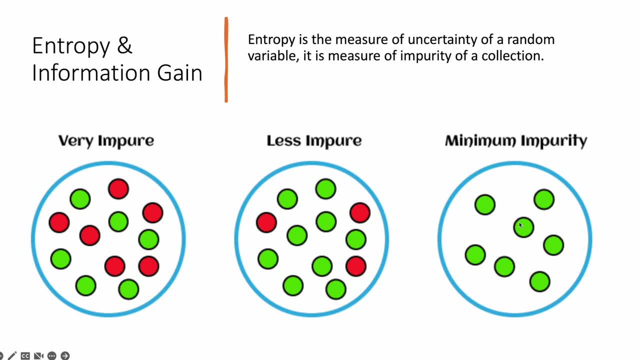 If either red or green, if only one class, would have been present. this is called minimum impurity or almost pure Right. This is the concept of entropy. In this particular case it's very impure highest entropy, This less impure medium entropy. 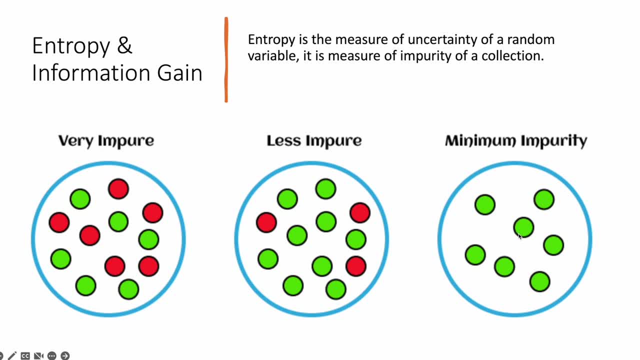 This is low entropy situation because only one class is present. If there is a mixture of both the classes in equal quantity, That is the very highly impure situation. This is the concept of entropy. What is information gain? We'll just see in a minute. 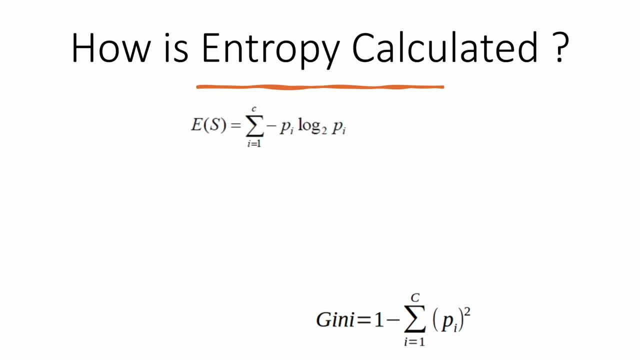 But first thing first, how is entropy calculated? And entropy calculated for categorical variables. How is entropy calculated? So this is the formula for calculating the entropy. right Now. this look formula may look complex, but let's break it down one by one. 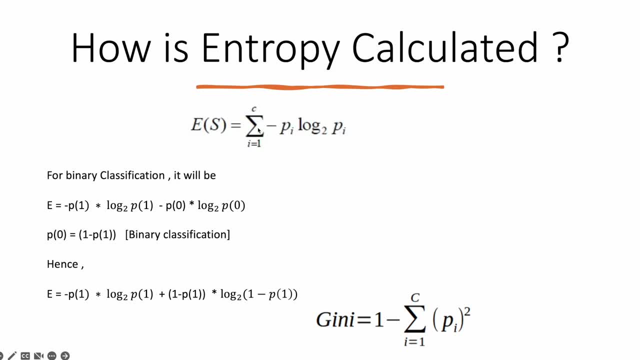 Okay. So the formula says: if there are C classes right Now, our problem is always binary classification. right, We have. we are splitting into two parts, right, Yes or no? Because our our, our. just for the understanding, let's say that we have binary classification. 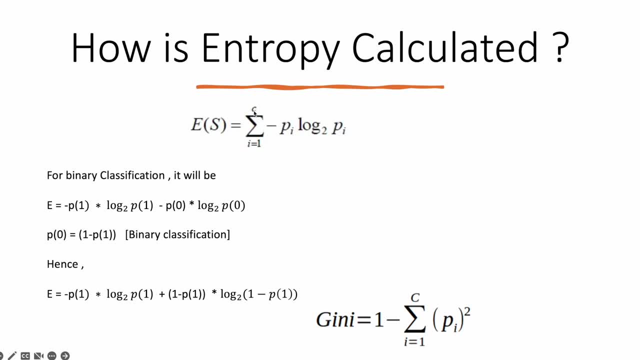 In that particular case, if we have to, C will become 2.. What will this thing become? This thing will become minus P, positive class. One is representing positive class. So minus P, log base 2: P1.. Again for my negative class. 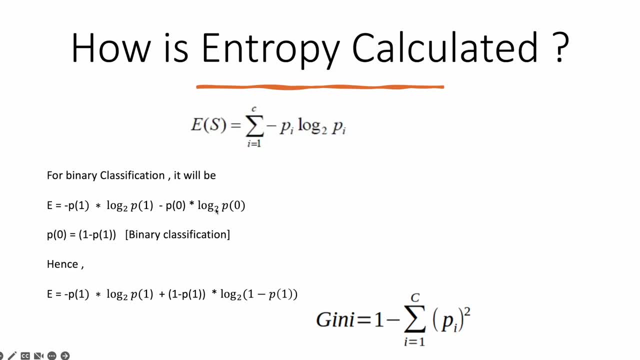 It will be minus P0, multiplied by log 2, P0, right, This is my the. the formula for entropy in case of a binary classification will be right. Now, in case of binary classification, friends, you already know that P0 will be 1 minus P1. 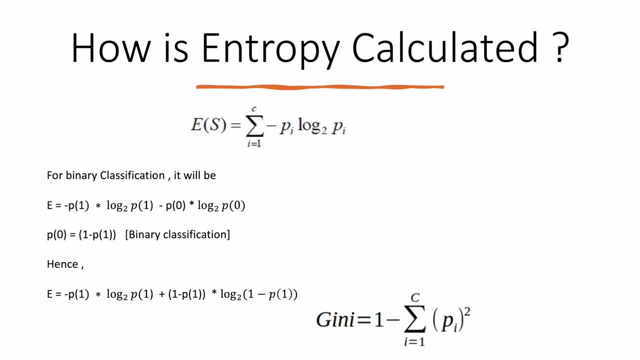 If the probability of getting a class- positive class- is 0.7.. What will be the probability of getting a negative class? 1 minus 0.7.. Which is positive, 0.3, right, So this formula also holds. 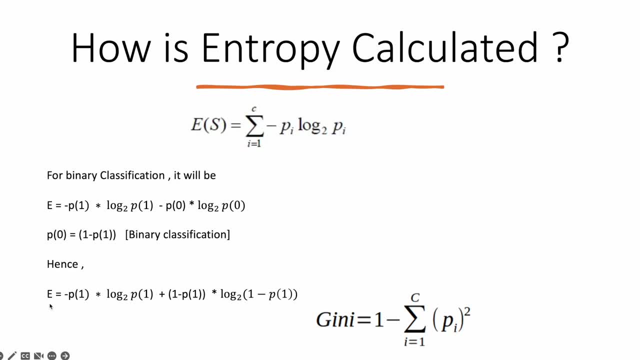 If we input this formula into this, we are getting this particular thing right. E is equal to minus P1. log base 2: P1 plus. we are just replacing this P0 with 1 minus P1.. That's all we have done over here. 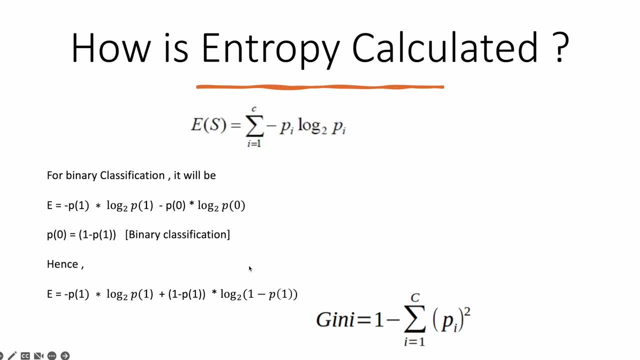 And this is the formula for binary classification. Okay, Entropy. Now one question will will come to mind. is that why we are taking this log of base 2 always in machine learning and mathematics we call natural log, Why we are taking 2 over here? 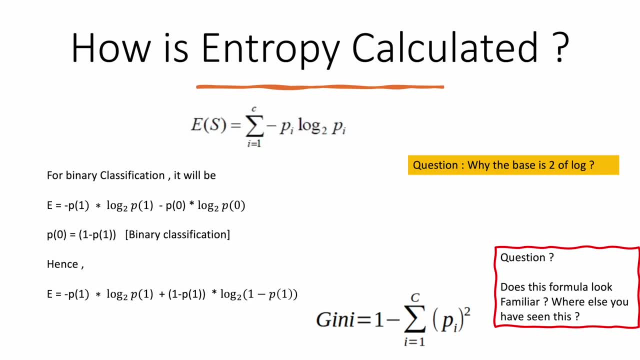 Okay, That's the first question, And the second question will come. is that, if you see this formula closely, it will resemble you to something right? Do you know where you have seen this? This formula you must have seen in case of logistic regression. 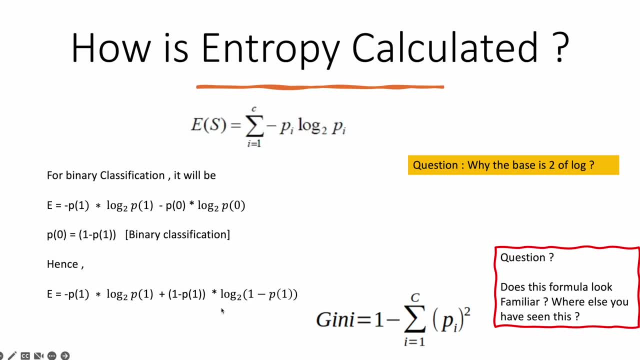 If you are doing a binary classification problem for a logistic regression, this formula will appear to you And that's why we call it over there binary cross entropy loss. If you recall and if you have not watched my logistic regression series video please, 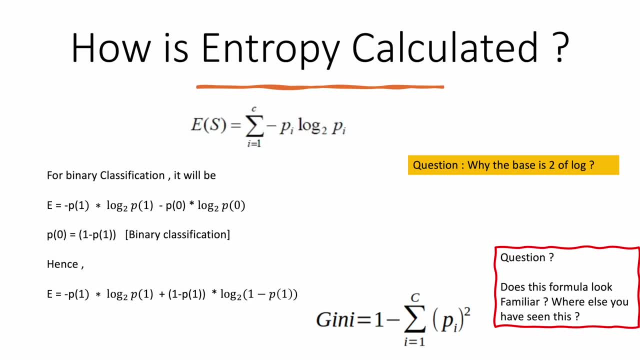 go ahead and watch that, You will understand that. Okay, So this is called binary cross entropy and it is used as a log loss function for logistic loss also. Now coming back to the first question, Why the base is log 2?. 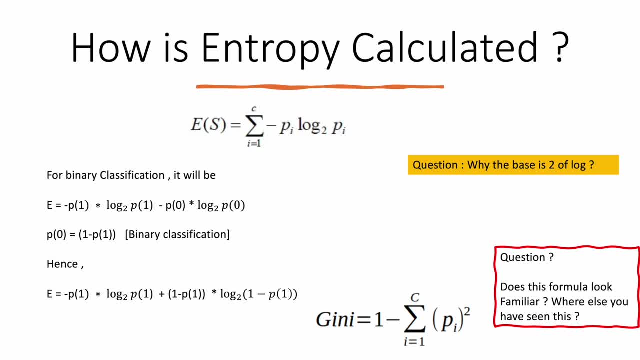 Now there is nothing essential over here, Like we are keeping base as log 2. Because the math does not. The math becomes more beautiful. Let's answer it that way. Okay, And why would that be? Let me show it with an example. 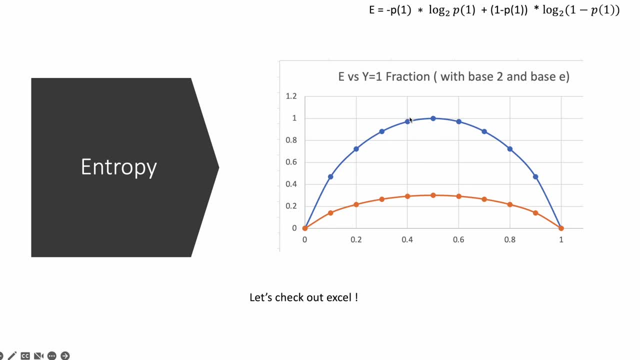 Okay. So what I am doing over here is I have plotted two graphs. Okay, This is a formula of E, right For various on the X axis. right Over here is the probability of your P1, right On the X axis. 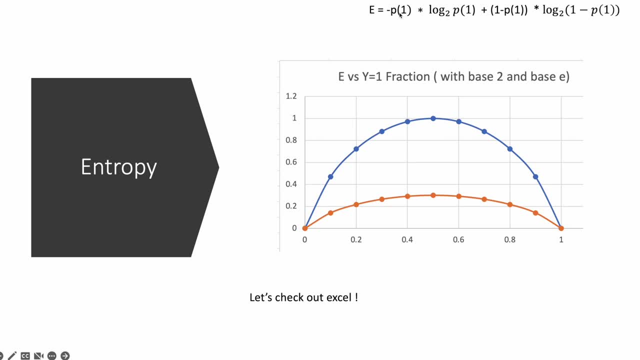 On the Y axis is my E or entropy. If I plotted this like for, let's say, P1 is equal to 0.1,, 0.2,, 0.3,, 0.4,, 0.5 till 1.. 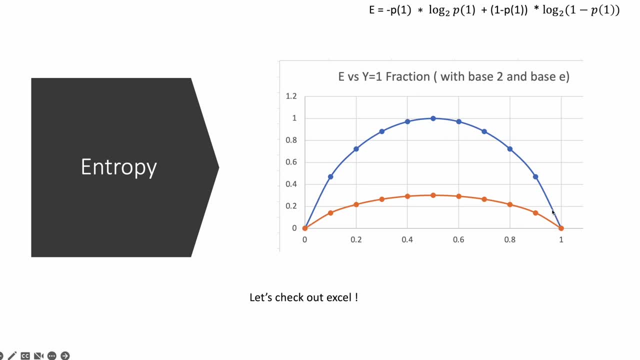 If I plotted, my graph looks like this: My blue graph represents the base 2.. If I plotted the same thing with log base natural number E, Euler's number, my graph is this: Okay, Now you will say that what is the difference between these two? 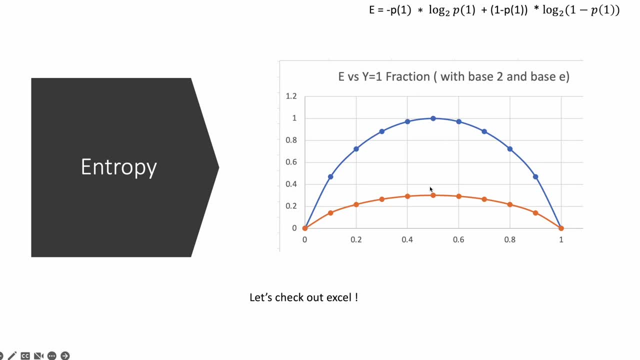 What is the difference between these two? Now, if you notice, this particular graph, which is the base of log 2, hits the maximum at 1, which is a nice round number matching with the probability, all those things. That's why we are using 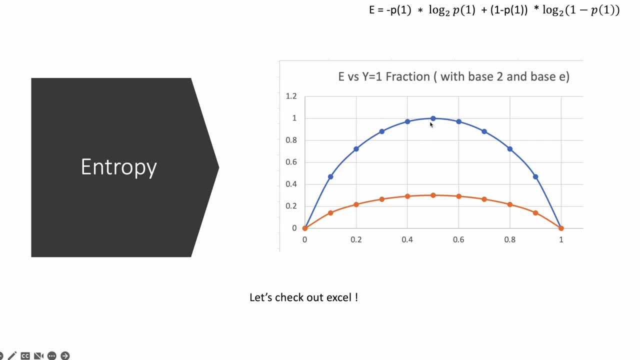 And why it is hitting, Why it is hitting at 1? Now let's see, It is hitting at 0.5.. Let's put 0.5 over here or half over here. Okay, So this particular term will be. 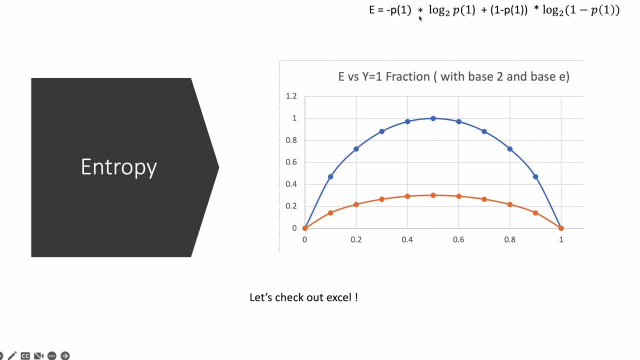 Will be minus half into log 2, half plus half into log 2, 1 minus half. Right, This will be the value. If you solve this value particularly, then you will come to know that the value of E which we are getting will be 1.. 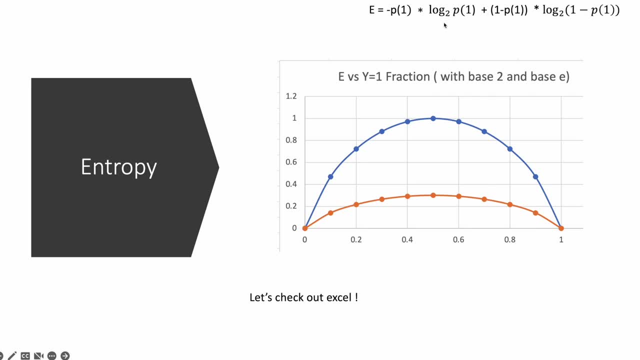 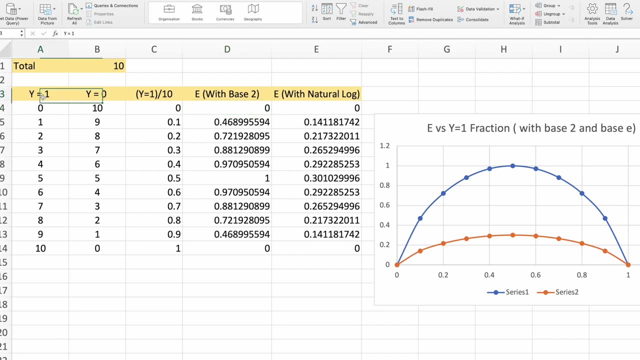 And that's why we are using the base of log 2.. Let's see that then. excel sheet also over here. Okay, This is the excel sheet. This is what I was talking about. What I have taken is over here is that my y1, y is equal to 0. 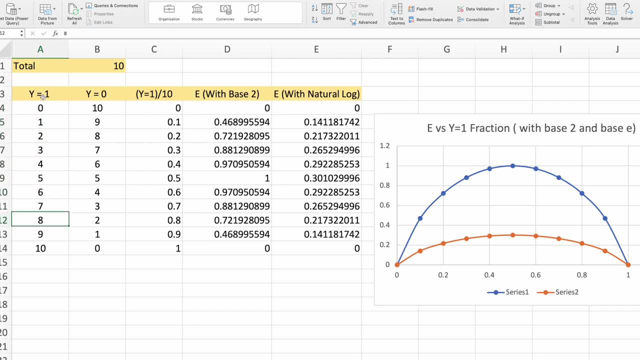 If y1 is equal to 0,, 1,, 2,, 3,, 4,, 5,, 6,, 7,, 8, and let's say there are 10 observations And for each category I am taking that let's say it is 0, and then my y is equal to 0, will. 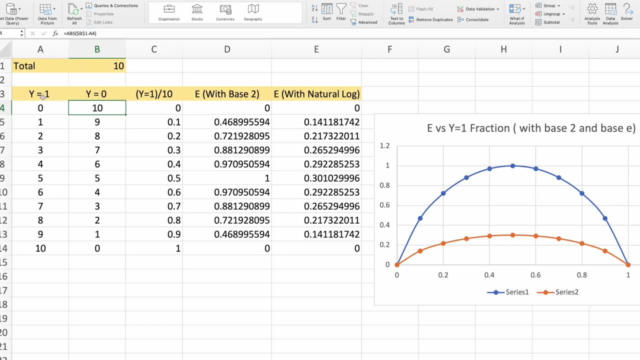 become 10.. That is because there are 10 observations. If my positive class is 0,, my negative class will be 10.. Positive class is 1, negative class is 9.. Similarly, I have drawn- and this is just to draw this figure- 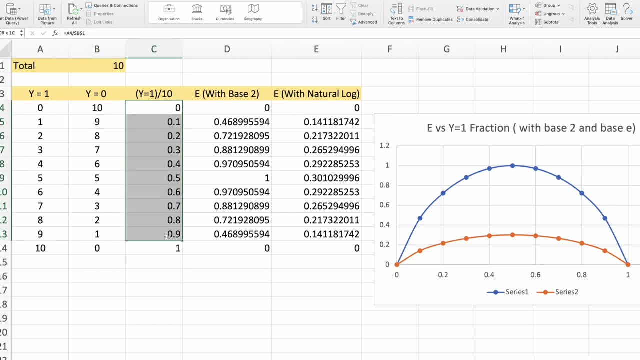 What I have done is I have calculated the p1.. This is by p1.. Right, How it is the p1?. This is nothing but this divided by 10.. Right, This is my p1.. The probability of getting positive class. 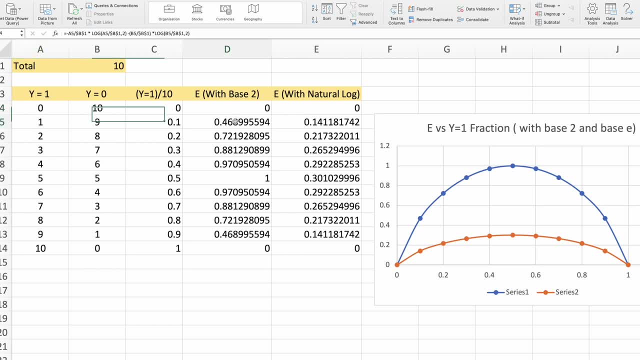 Now, with base 2, I have done the calculation. If you see, I have done the calculation with base 2.. With natural log also, I have done the calculation. If you notice, these numbers are very symmetrical. Right Across this y axis this number will be very symmetrical. 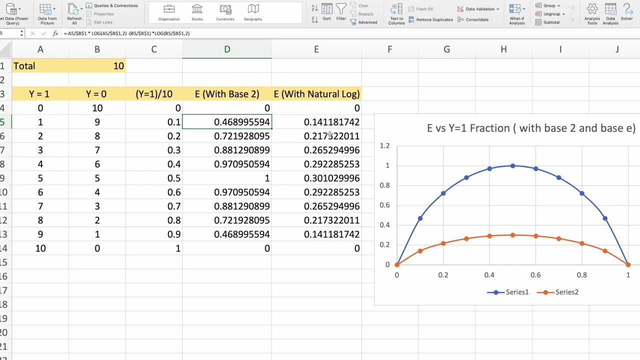 Right, It makes sense With natural log also. I have done that Now if you see the blue line actually touches at the 1.. Right, If you see over here, when the probability is half, that my positive class and negative class are equally likely, 5, 5.. 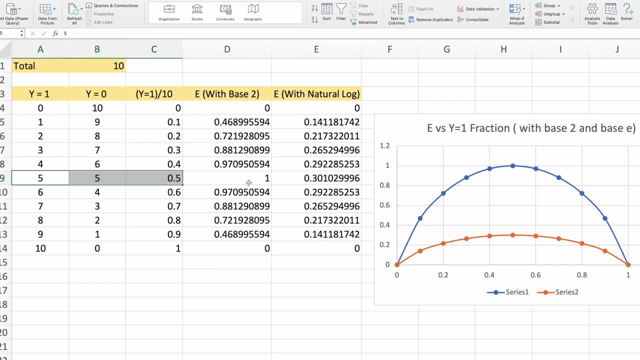 My probability is half of p positive class and half of p negative class. What is the value of entropy which I am getting? I am getting a nice round number 1.. But at the same, what is the probability I am getting? 0.30.. 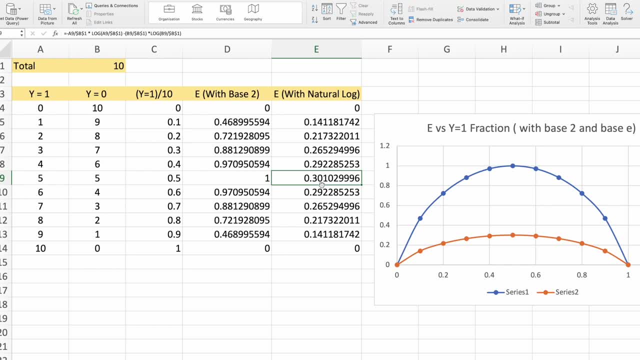 Which is not very nice and wrong. That is why- that is the only reason why we are using the base of log 2 instead of base of log e. There is no reason. It is just that it will be a different curve, Right. 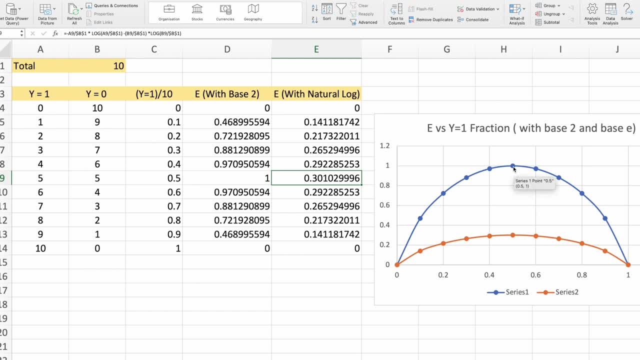 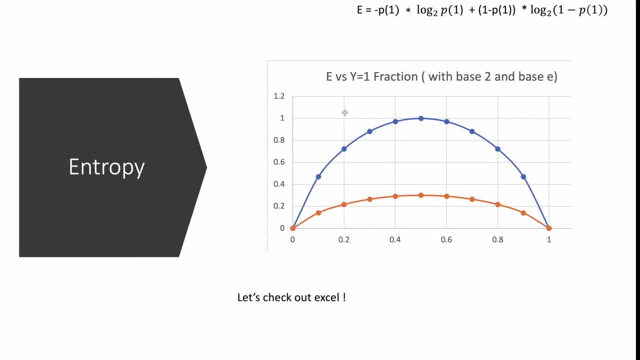 It will still solve the problem, But this looks much more cleaner and beautiful, Right, Ok, Now the other thing to notice over here is: let us go back to our slide. Yeah, Other things to notice over here. If you input log 0.. 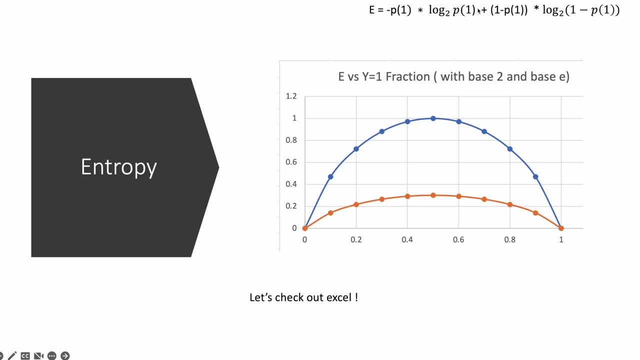 If you calculate the value of 0. What will be this particular thing, p1.. If log of 0 is actually undefined, Right, But for the practical purpose of calculating this, p1 is equal to 0. Then log 0.. 0 into log 0. 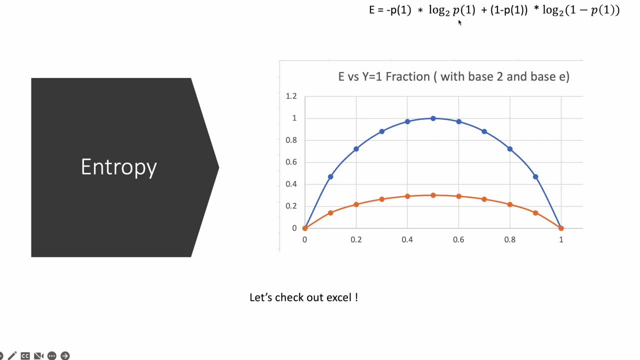 So we are considering this whole element as 0, not as undefined Right. So this is a small assumption which we are making to ensure that this is meeting at 0 and 0.. Right Over here, At both at 1 and at 0, our entropy becomes 0. 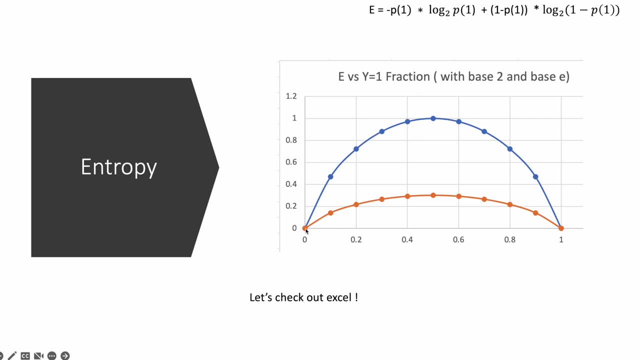 Right Entropy becomes 0. means what? Let us try to understand what this 0 and 1 means. At probability 0 also, there will be only and only negative class. At probability 1, it is only and only positive class. Ok. 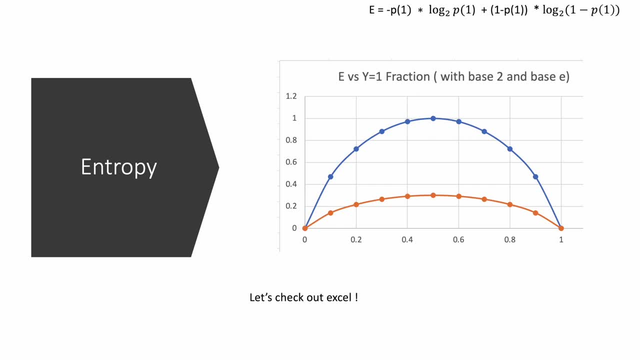 So remember that ball. If there is only negative class or only positive class, What will be my impurity? It will be very pure, purest form Right, And my entropy will be the lowest Right, Because entropy is a measure of impurity. 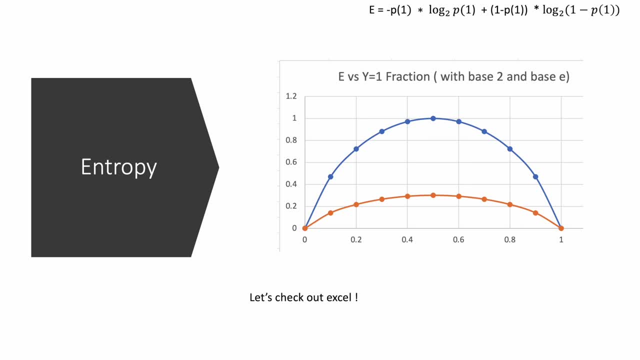 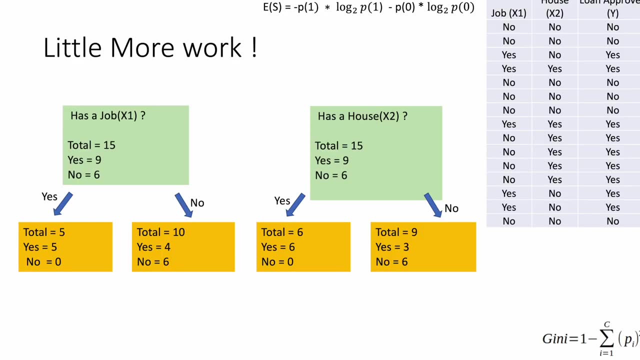 So my entropy will be close to 0 or almost 0. Right, So this figure makes intuitive sense to you. Right To understand what entropy means. Now coming back to our original problem, where we are doing the splitting and partitioning Right. 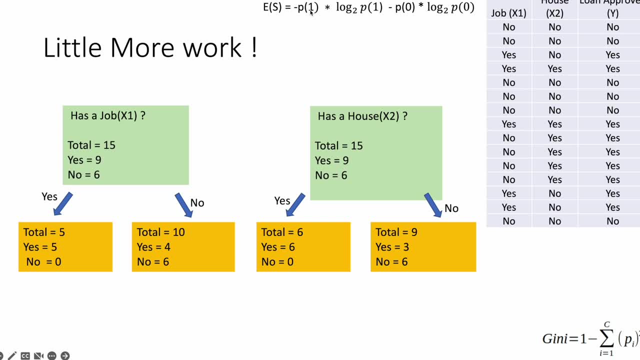 And this is the formula to calculate the entropy. Just remember that for a binary classification problem. Ok, Now let us see what we are doing over here. We are trying to create using this formula. We are trying to create the entropy, Ok. 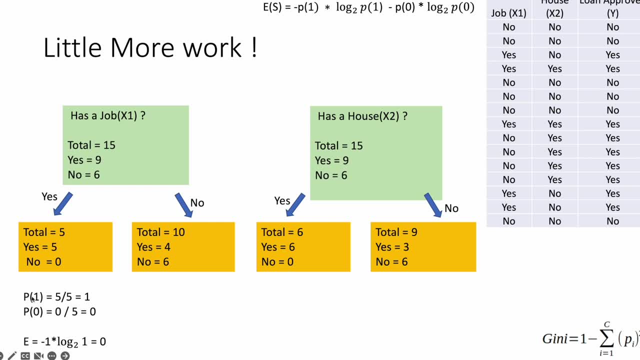 We are trying to create Now. Now, what will be the p1?? Because yes was 5.. There were total 5 observations, So 5 by 5.. 1 is p1.. Positive class: p0.. There was 0 negative observation or negative class or 0 class. 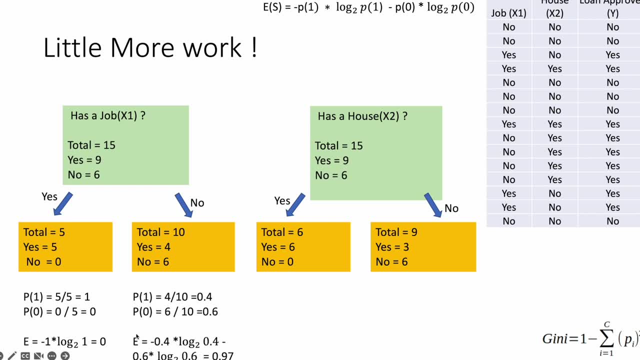 0 by 5. 0.. Similarly, we will calculate E or entropy for each of these combinations. Ok, So all the 4. I have calculated the entropy And what I have received: 0.. 0.97.. Again, entropy is 0 over here. 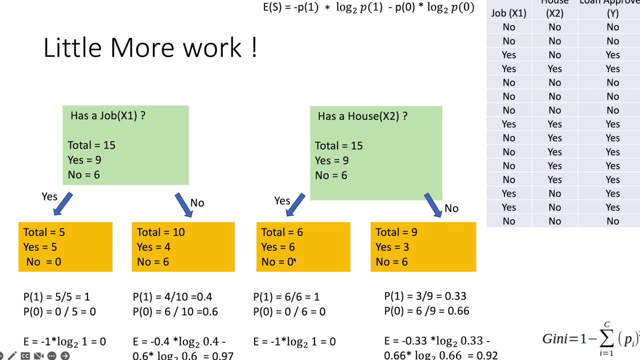 Because it is. It is almost pure, solid, Pure mixture. Right, Because it is only one class. Obviously, the entropy will be 0.. Right Over here also, the entropy is 0.92.. Similarly, we have to calculate the entropy for our root node also. 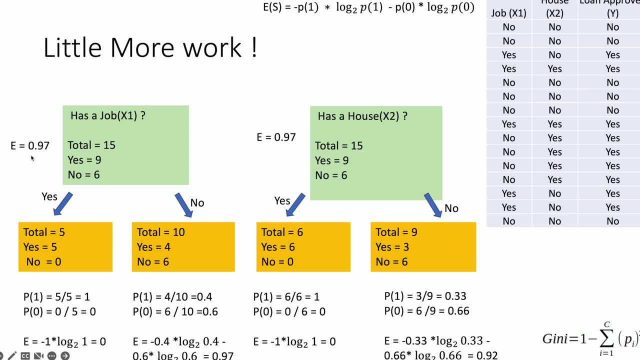 So the entropy for root node is 0.97. Entropy. obviously there were 15 things or observations. 9 of them were yes, 6 of them were no. What is the entropy? We just put it in the formula. We got it. 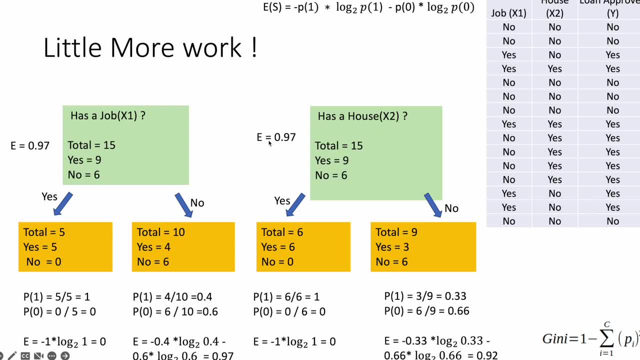 Right 0.97.. Here comes Now. we have understood what is entropy. Let's also understand what is information gain. Information gain means how much entropy we were able to reduce. The reduction in entropy is called information gain. So entropy at root node was this. 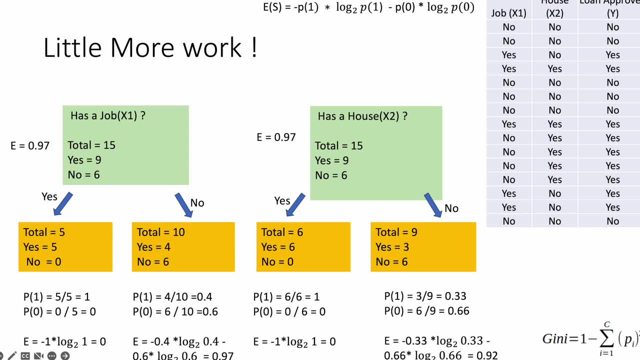 Entropy at child node is 0 and 0.97.. If we do this particular split, The entropy at root node is 0.97.. And entropy at child nodes are 0 and 0.92.. Now, friends, the question is: our last function was entropy. 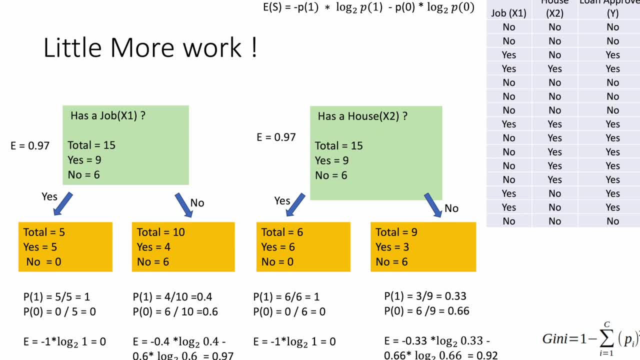 We have to reduce the entropy. In other words, what we have to do is the reduction in entropy is also called information gain. So we have to maximize the information gain. That's fine, But the question is over here: 0.97.. One node is 0.. 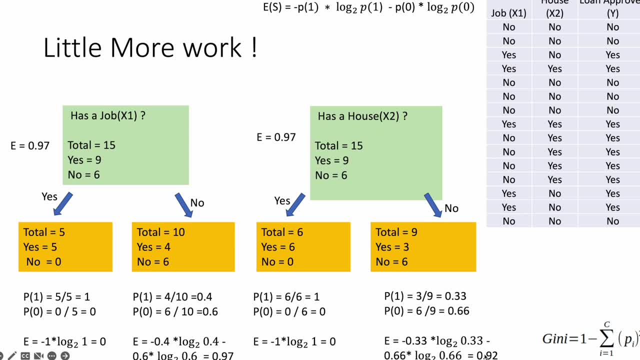 One node is 0.97.. 0.97.. One node is 0.. One node is 0.92.. Which split is better? Still, there is no way of knowing which split is better, Right? So let's try to dig more. 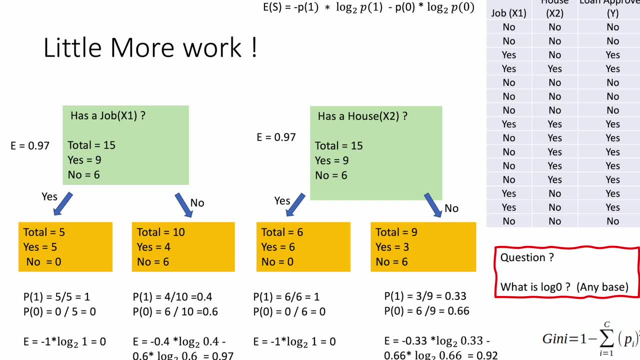 Right, What we will do is Okay This: I have already answered that. why log 0.? Right, If you take log 0. We have just discussed that. any base it is called undefined, But for this purpose we will assume that it is 0.. 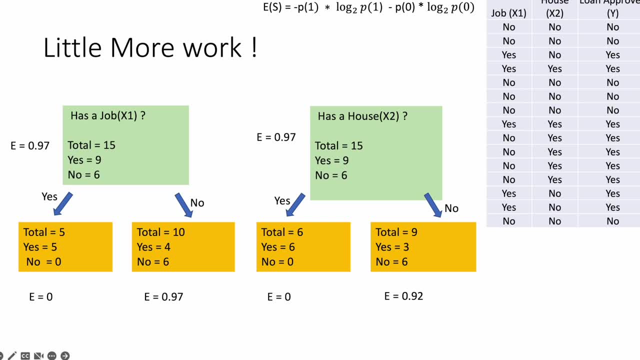 Right, Okay, Now We have removed all those And we for all these yellow blocks or splits, or the child entries. We have just wrote down what the E which we got Right. We have little more work to do, So pay attention. 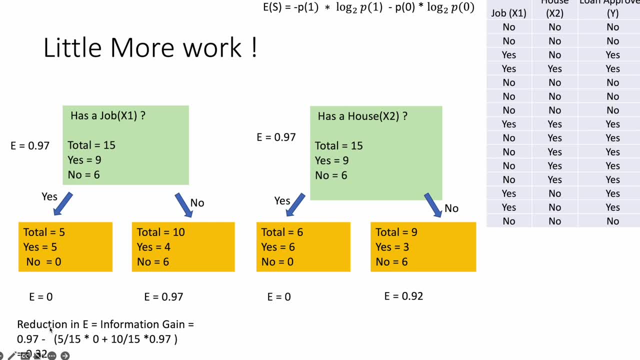 What we will do is What will be the information gain. Information gain is nothing but reduction in E. Correct How we calculate the reduction in E. The E at the root node was 0.97.. Then we will take a weighted average of the entropy at both the nodes. 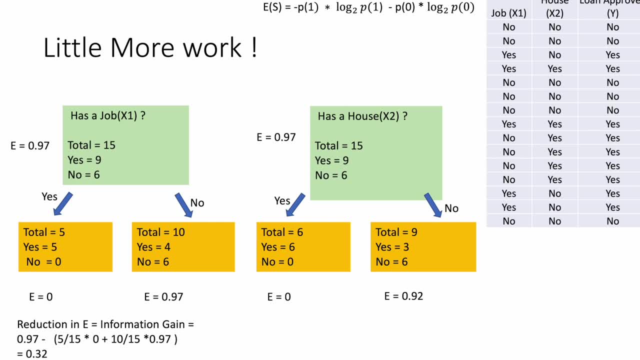 Right, That would be the right thing to do. Think intuitively why it would be. Because this thing has been split into 0 and 0.97.. Here, 5 observations have gone. Here, 10 observations have gone. Right, We cannot just take that. 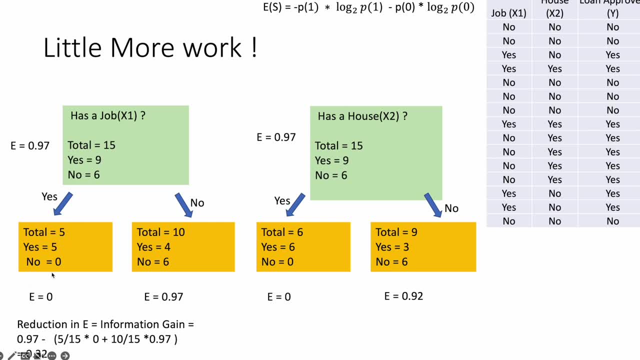 Okay, Based on 5 observations, this has become very pure, So let's go with this. No, We have to find a mechanism where we have to give weightage to how the split is happening, Or what is the weight of the split. also, 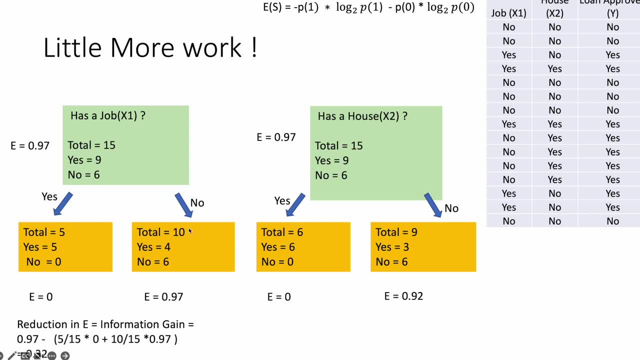 Suppose there is just one observation here And 14 observations over here, Should we consider both of them reduction equal? No, It should be weighted Because the reduction in entropy is also related to how many observation. based on that we are calculating Right. 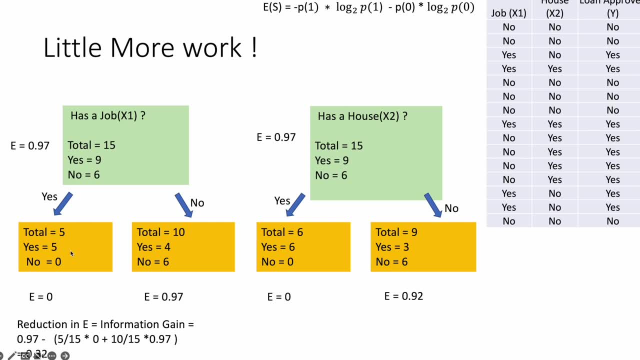 So what we are doing is: Out of 15 observations, 5 is over here Out of 15.. 10 is over here, So 5 into 15, multiplied by entropy. at this point, Entropy at this level, Again, weight. 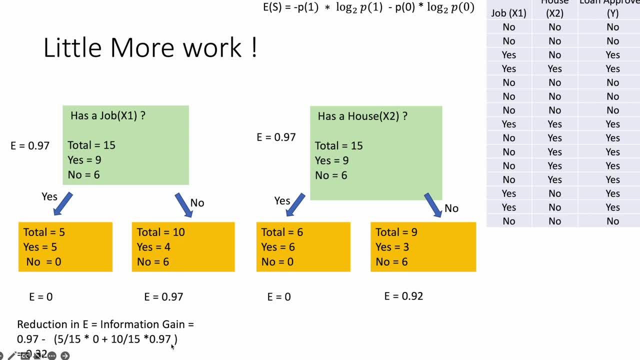 What will be the weight of this? 10 by 15 into 0.97.. This is the total entropy. This thing, within parenthesis, Is the total entropy of the child. And what will be the reduction of entropy? The parent Entropy of parent minus entropy of child. 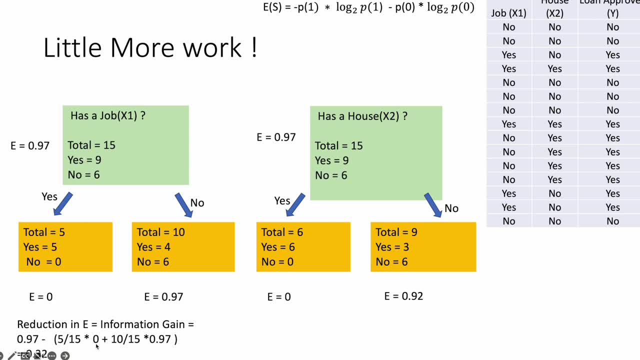 Entropy of parent minus entropy of child Right. Similarly, we will calculate it over here. So over here, if you see, it is 0.32.. Over here, it is 0.38.. Now, Now you tell me That where the information gain is more, 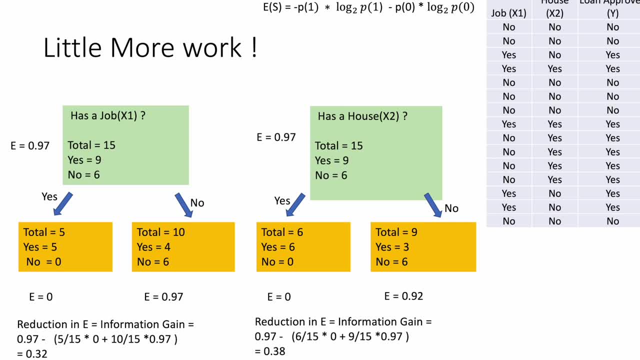 Or the reduction in entropy is more. They are both the same thing. Information gain is nothing but the reduction in entropy. The reduction in entropy is more on my right split, Based on the house. So this will become my root node, Because my entropy is. 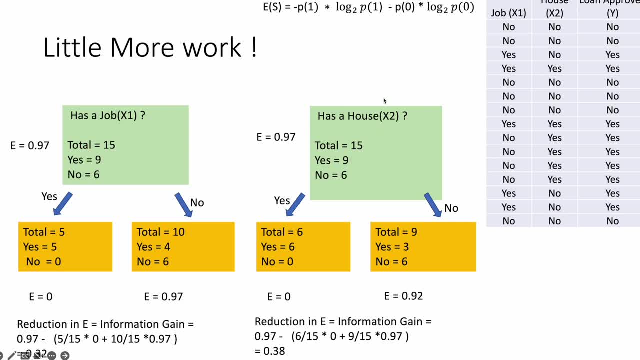 The reduction in entropy is highest at this split. Again, friends, If there are multiple features, You have to repeat this exercise for all the features, Because every feature will be a candidate for split At the root level. Which one you are selecting? 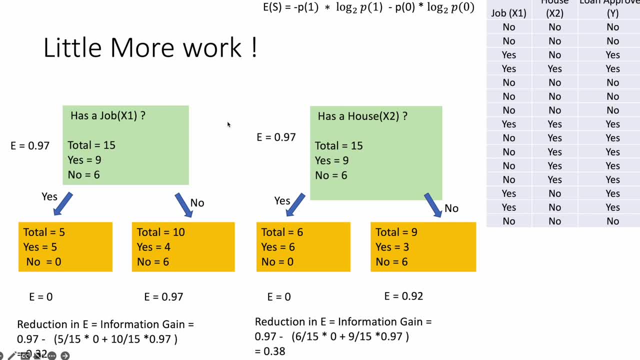 Is based on this: calculating the entropy, Calculating the reduction in entropy Or information gain, And then selecting the one Which has the highest information gain Or the highest value of reduction in entropy. Clear. So I have to do my base split. 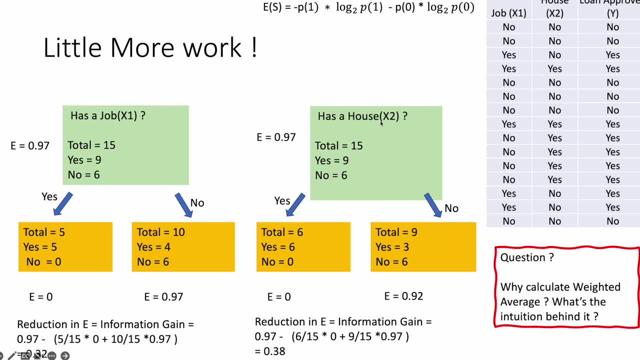 Or the root split As at house level. Correct? This is how we do that. Now why calculate the weighted average? I think I already told you It makes sense logically also to do it, Because suppose there is just one observation And 14 observation over here? 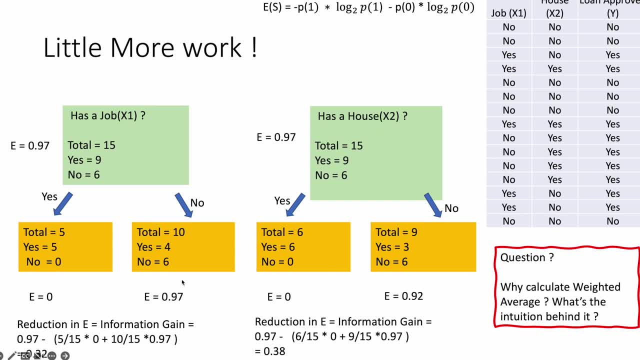 We should not take the average of entropy, Right. That will not make sense Because most of the observation has gone over here. So we should give due weight to that particular scenario also, Right, Okay, That is why. That is the intuition behind. 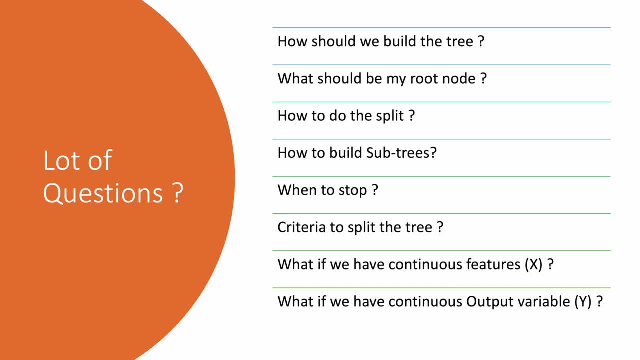 Still, we have lot of questions. Right, We initially saw those questions that how should we build the tree, What should be my root node? I think we partially answered that. We answered that: what should be my root node? Right, We also answered that: how we build the tree. 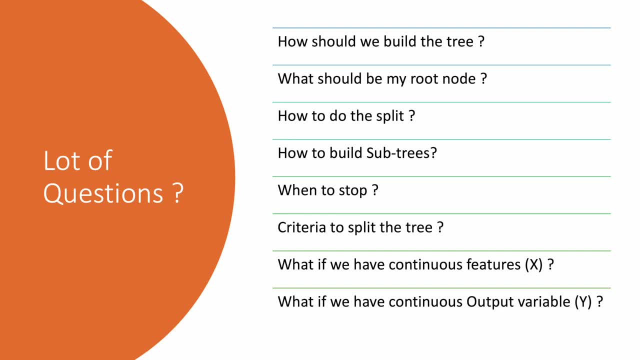 How we do the split, at least at the base, at the root node. We already know that. How do we build the sub tree? These are the some of the questions which are still. When to a stop. When I reach? How will I know that I have reached the leaf node? 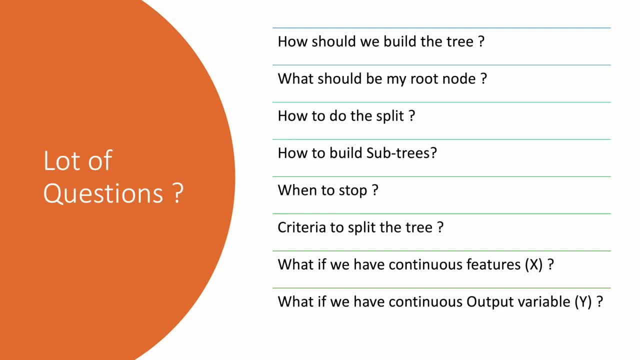 These are the questions which are still pending. Okay, We will see these questions in my second video. Till then, have a good day. Bye.